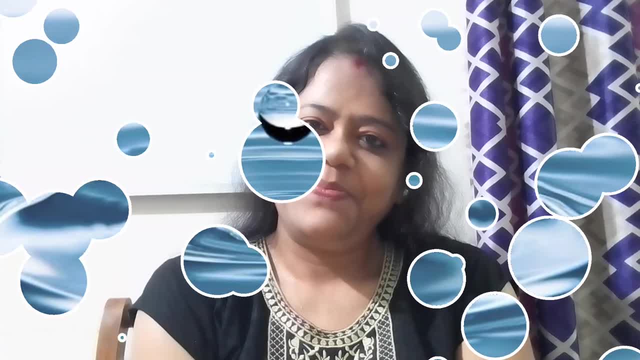 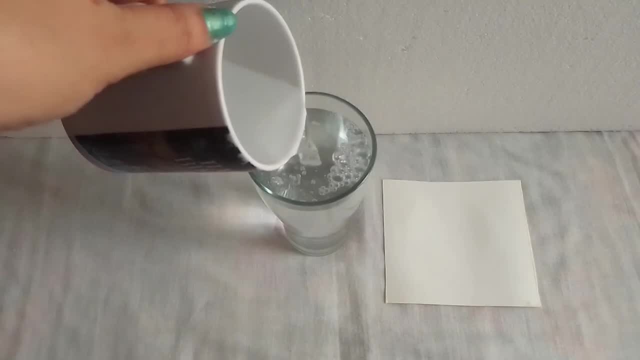 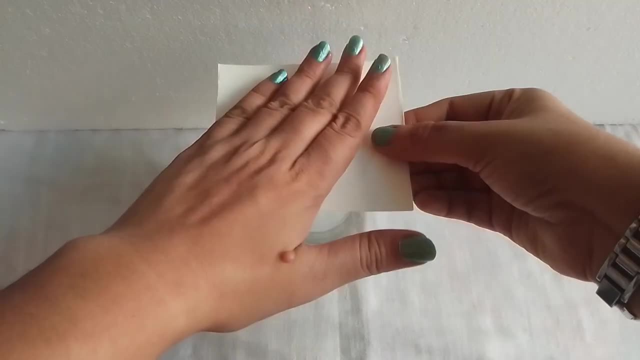 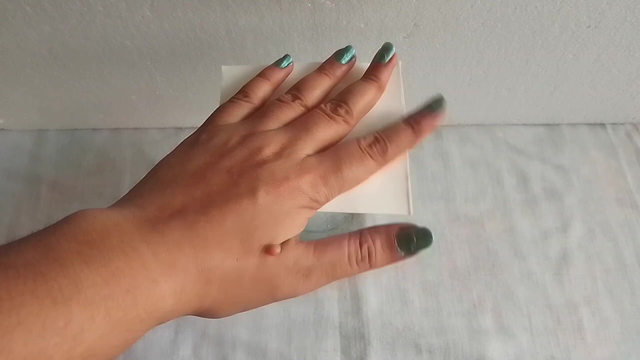 So let's get started. Here is a glass and a paper and I am filling water in the glass full of it. Now I am covering the glass with a piece of paper and I am little bit pressing it, and now I will try to move the glass upside down and let's see what will happen. 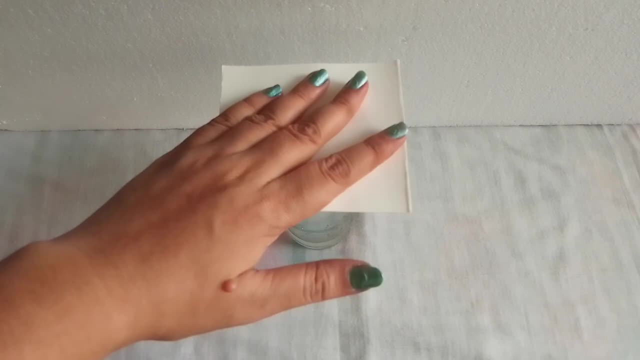 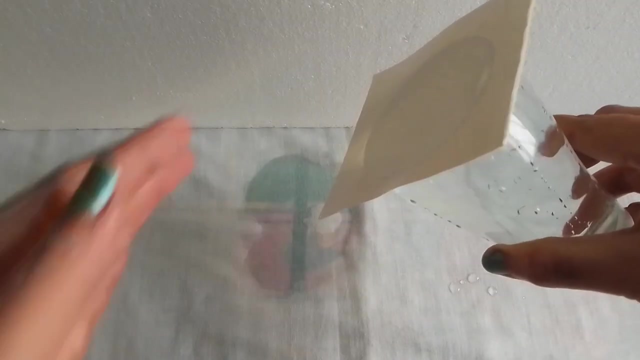 In this experiment, the water in the glass pushes the glass. It pushes the air out of the glass, so there is no air pressure inside the glass. Now, slowly, I am making it upside down and you can see that water also not falling down and the paper piece also not falling down. 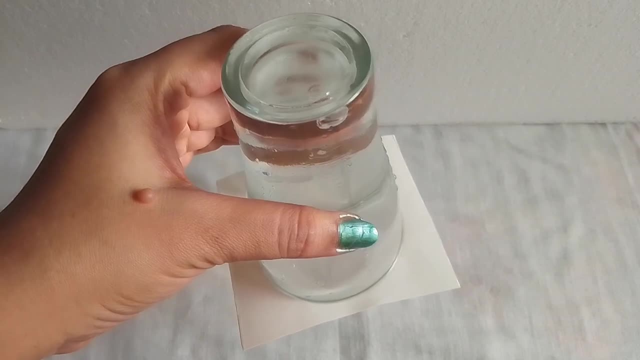 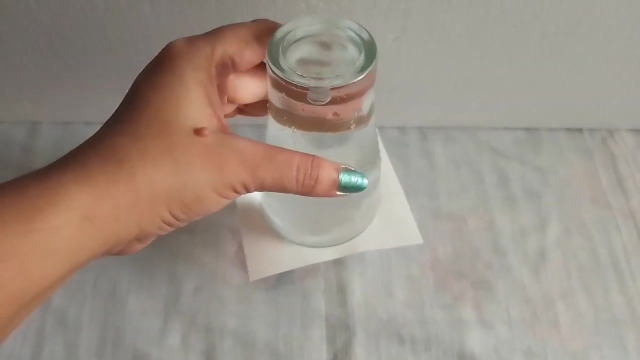 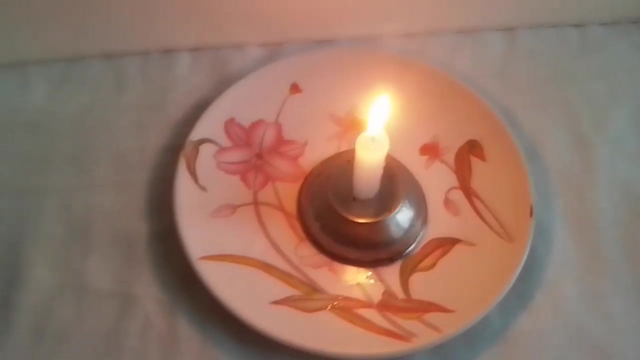 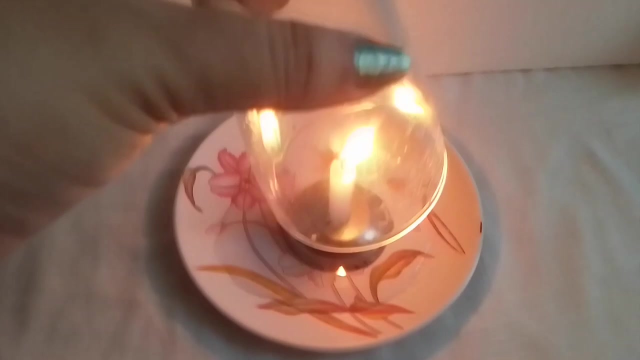 Why? Because air particles can move freely, so the atmospheric pressure pushes on the glass from all directions, holding the paper in its place without water falling out of the glass. In my next experiment, on a plate I kept a burnt candle and I am putting water outside the candle on the plate and slowly I am covering the burnt candle with a glass. 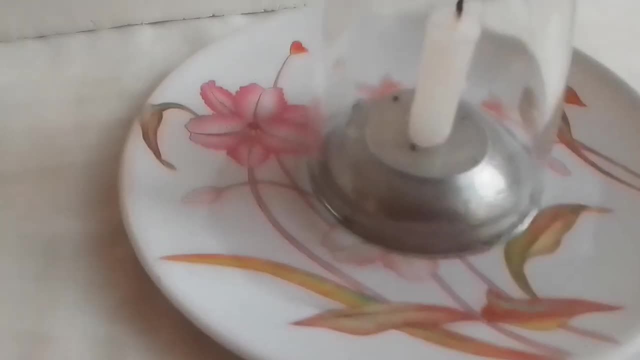 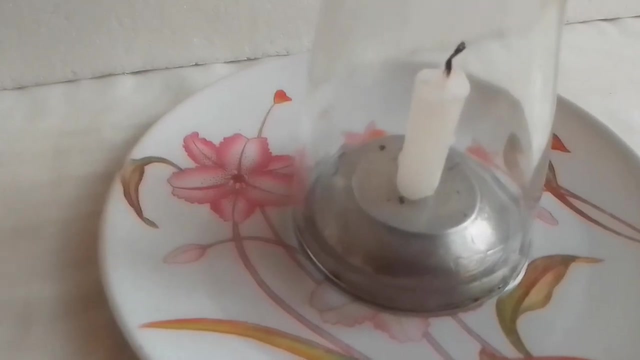 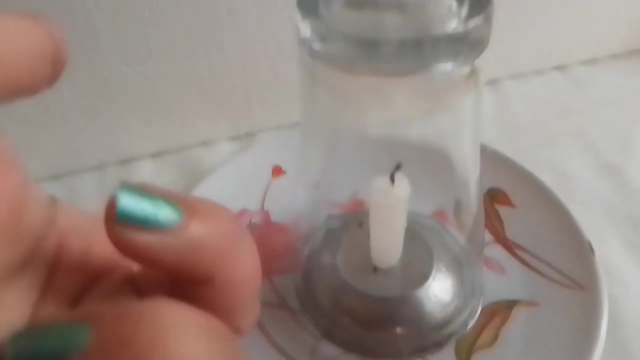 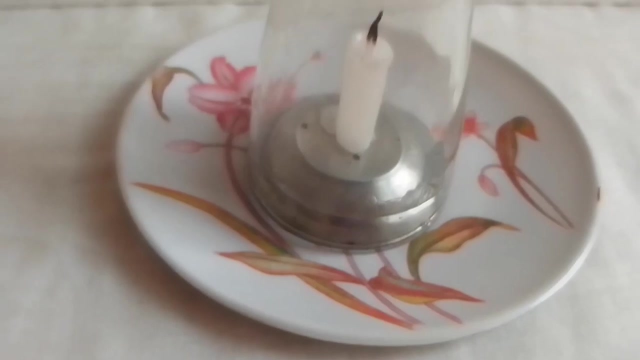 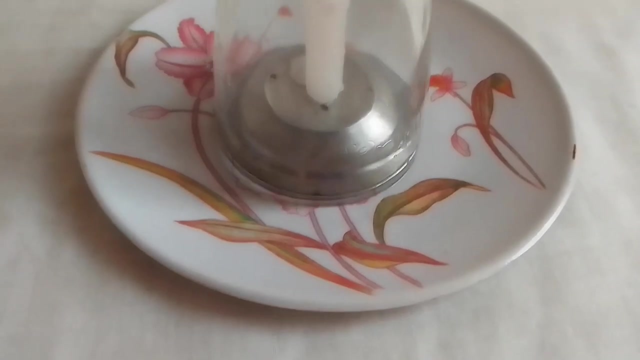 So see what is happening slowly. slowly the candle dimmed and then it is put off. Now you can see that slowly the water of the plate is coming inside the glass. Why it is happening? because the burning candle consumed the oxygen inside the glass, so there is partially empty place and to fill up this empty place, the water is coming up inside the glass. 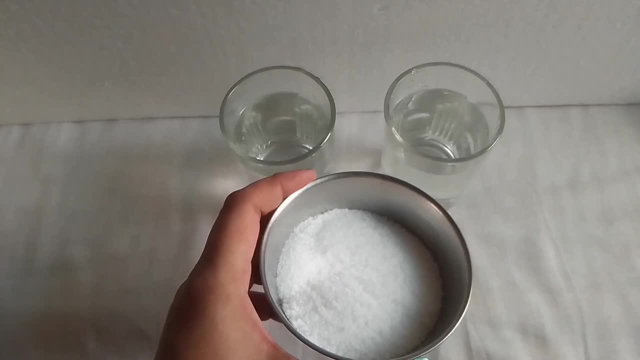 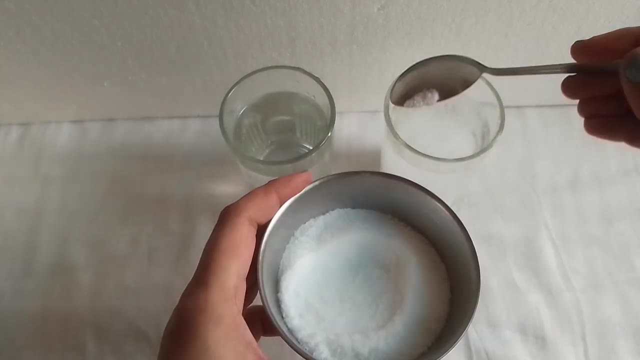 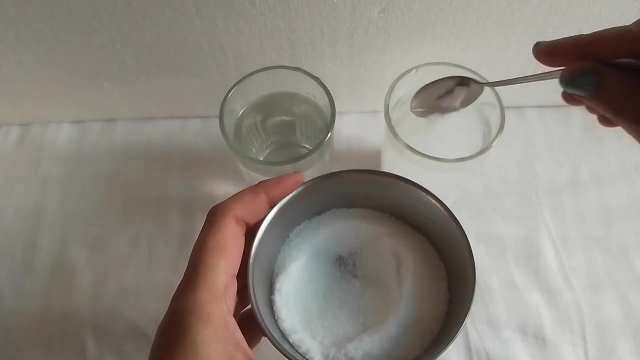 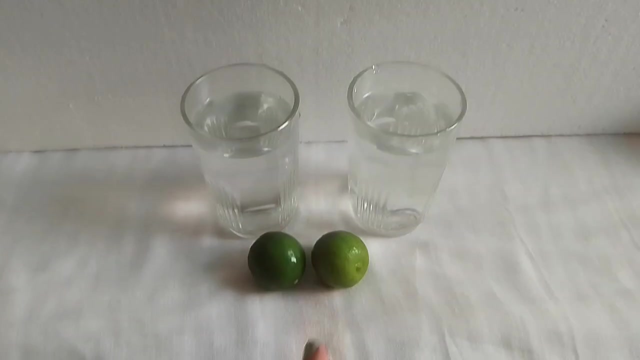 In my next experiment I have taken two glasses of normal tap water and in one of it I am putting two teaspoons of normal table salt and I am stirring well until the full of the salt- the total salt- is dissolved in the water. Now the right side glass is salt water here and the left side glass is normal water here.